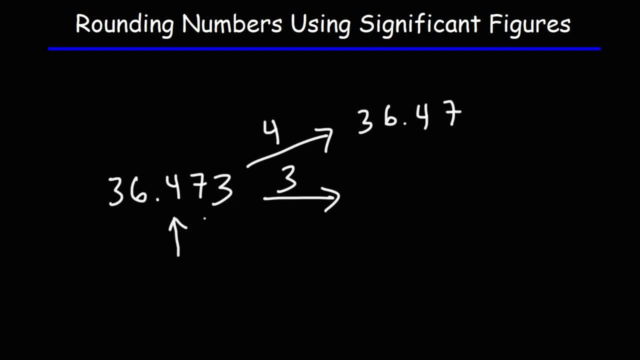 So 4 is the third significant digit. Looking at the number to the right of 4, we have a 7.. 7 is 5 or more, so we're going to round a 4 up to a 5.. So this is going to be 36.5.. 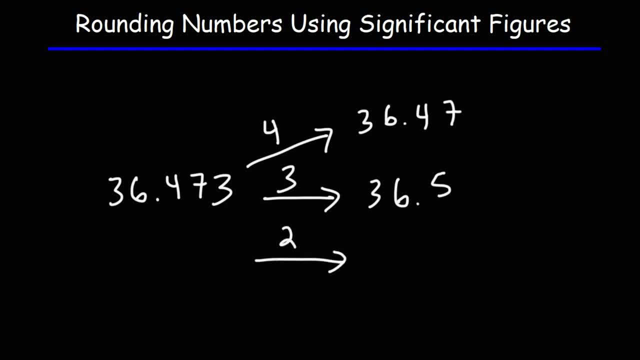 Now what if we want to round that same number to two significant figures? What would the answer be now? So 6 is the second significant digit. Looking to the number to the right of 6, that's a 4.. So that's not 5 or more, which means we're going to round down. 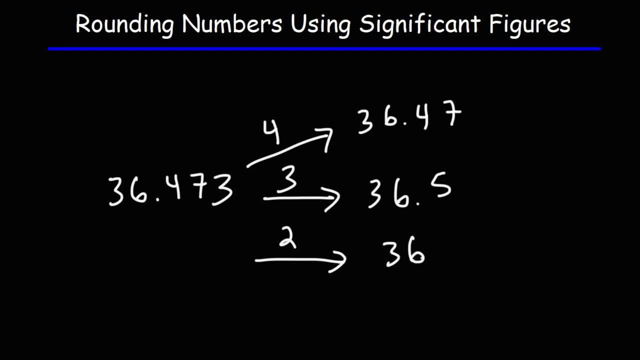 So 36.5.. So 36.473 will be rounded to 36.. Now, finally, what if we want to round it to one significant figure? In this case, let's focus on the first significant digit, which is a 3.. 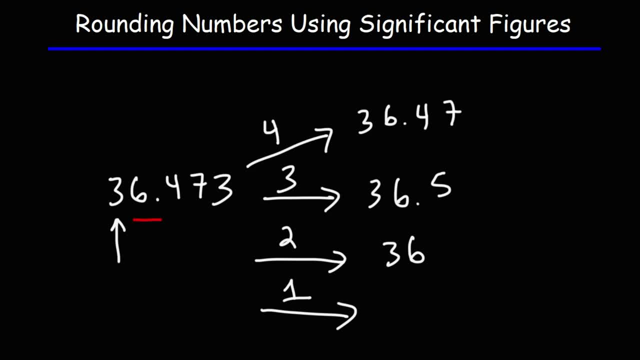 Focusing on the number to the right of 3, we have a 6.. So that's in the category of 5 or more, which means we're going to round a 3 up to a 4.. So 36.473, we're not going to round it to 4.. 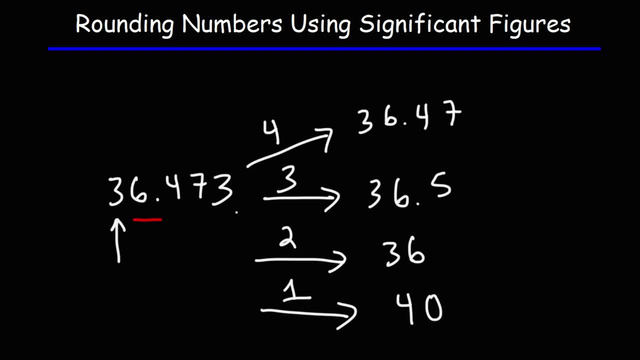 We're going to round it to 40.. 40. It's closer to this number than 4 is Now 40, this doesn't have two significant figures. This has one significant figure, A 0, that exists to the right of a significant figure like 4, that doesn't have any decimal points. that 0 is not significant. 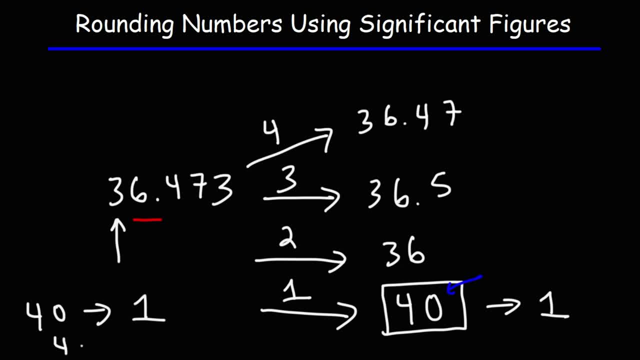 So 40 has one significant figure, but 40 with a decimal point has two significant figures. Again, you can learn these rules In that video entitled Significant Figures- a Fast Review. So you can find that in the description section below this video. 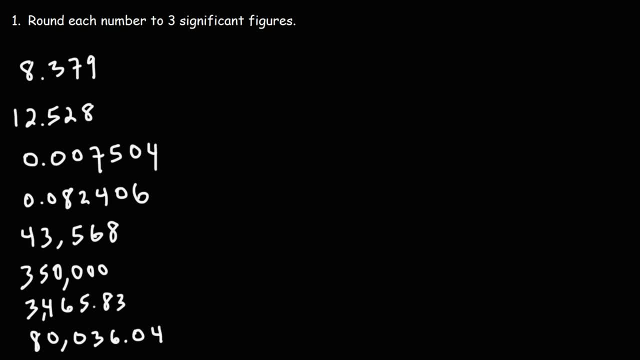 Now let's work on some practice problems. Round each number to three significant figures. Feel free to pause the video if you want to work on these problems yourselves. So let's go ahead and begin. 8.379, how can we round that to three sig figs? 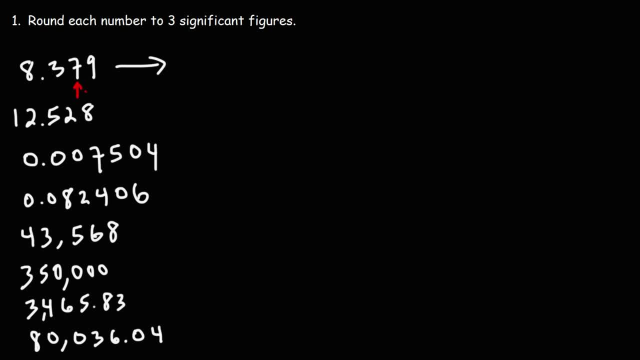 So let's focus on the third significant digit, from the left, that's a 7,. looking at the number to the right, that's a 9, so that's part of the category of being 5 or more. so we're going to round the 7 up to an 8.. 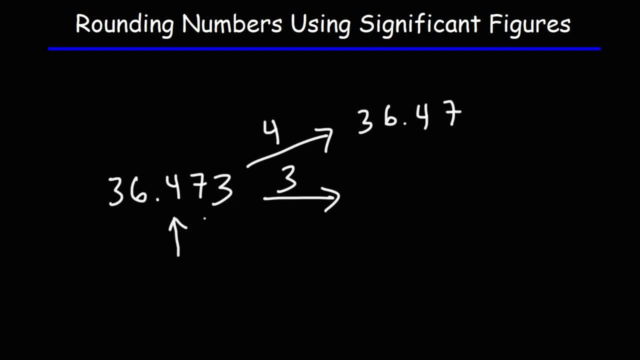 So 4 is the third significant digit. Looking at the number to the right of 4, we have a 7.. 7 is 5 or more, so we're going to round a 4 up to a 5.. So this is going to be 36.5.. 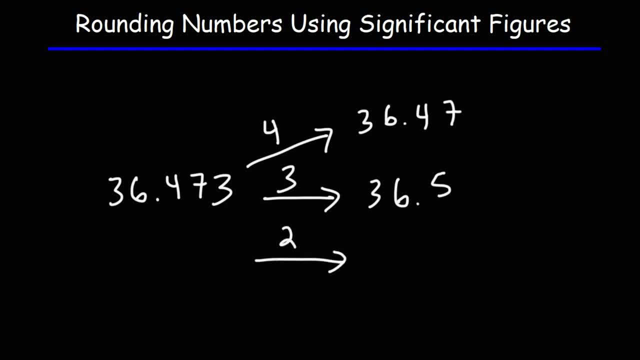 Now what if we want to round that same number to two significant figures? What would the answer be now? So 6 is the second significant digit. Looking to the number to the right of 6, that's a 4.. So that's not 5 or more, which means we're going to round down. 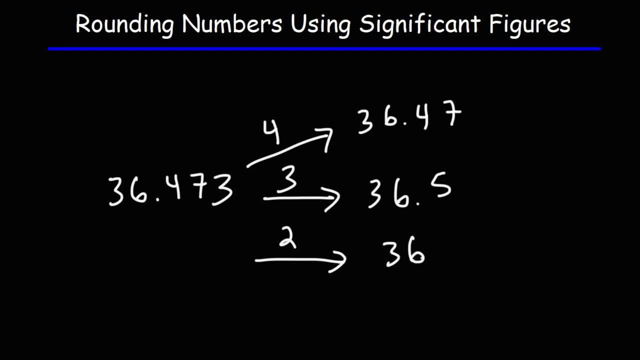 So 36.5.. So 36.473 will be rounded to 36.. Now, finally, what if we want to round it to one significant figure? In this case, let's focus on the first significant digit, which is a 3.. 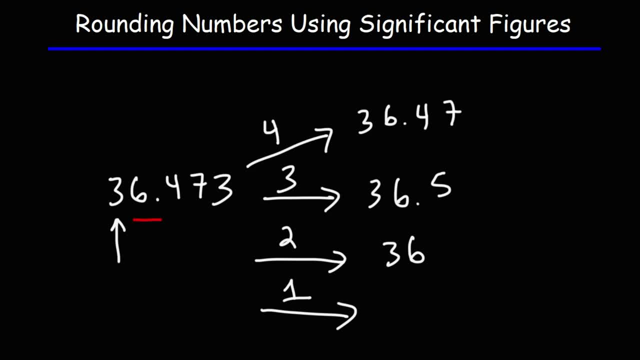 Focusing on the number to the right of 3, we have a 6.. So that's in the category of 5 or more, which means we're going to round a 3 up to a 4.. So 36.473, we're not going to round it to 4.. 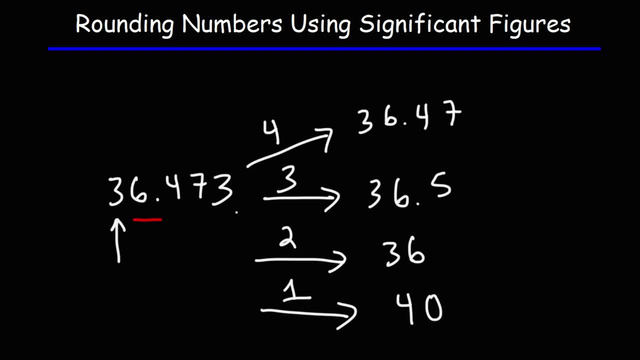 We're going to round it to 40.. 40. It's closer to this number than 4 is Now 40, this doesn't have two significant figures. This has one significant figure, A 0, that exists to the right of a significant figure like 4, that doesn't have any decimal points. that 0 is not significant. 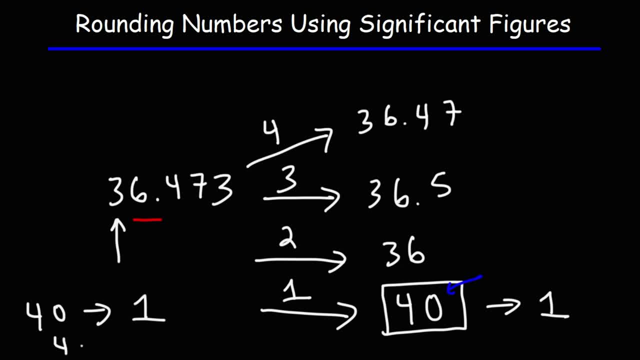 So 40 has one significant figure, but 40 with a decimal point has two significant figures. Again, you can learn these rules In that video entitled Significant Figures- a Fast Review. So you can find that in the description section below this video. 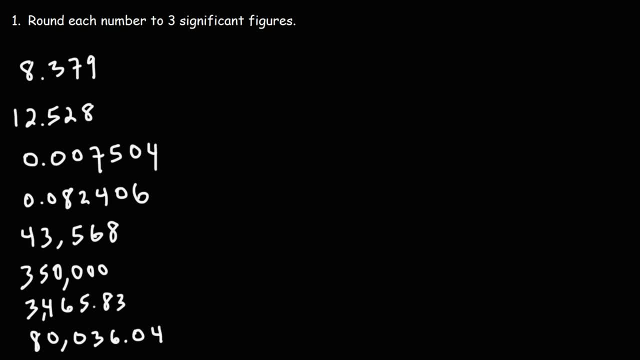 Now let's work on some practice problems. Round each number to three significant figures. Feel free to pause the video if you want to work on these problems yourselves. So let's go ahead and begin. 8.379, how can we round that to three sig figs? 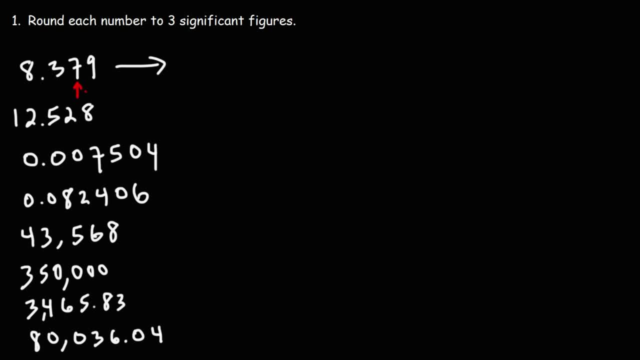 So let's focus on the third significant digit, from the left, that's a 7,. looking at the number to the right, that's a 9, so that's part of the category of being 5 or more. so we're going to round the 7 up to an 8.. 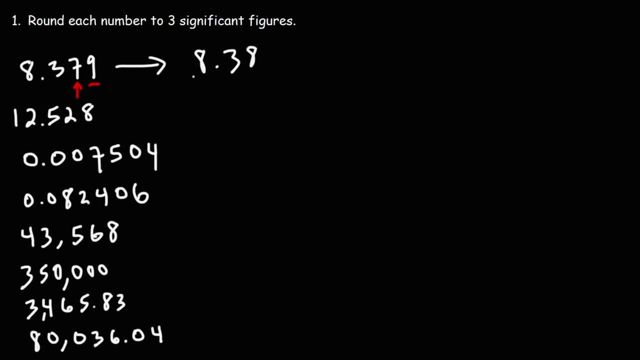 So this is going to be 8.38.. And this number has three sig figs, so we could stop here. Now, what about 12.528?? So we're going to focus on the third significant digit. Looking at the 2, that tells us that we need to round down. 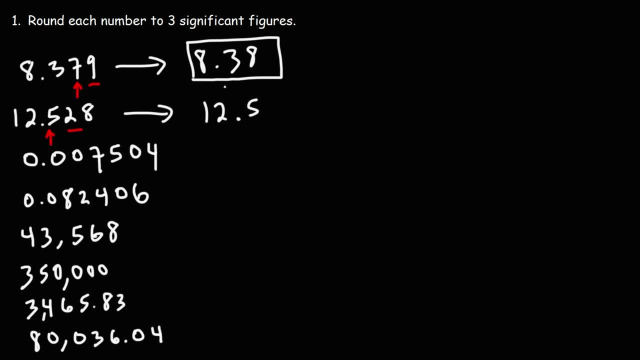 So we're going to round 12.528 to 12.5.. So this number has three sig figs. Now what about .007504?? Now you need to know that zeros to the left of the first significant digit, these zeros are not significant. 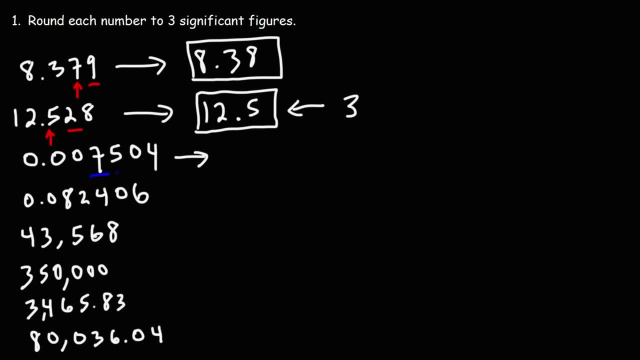 So this is the first significant digit. this is the second one. A zero between two non-zero numbers. that zero is significant, So this zero is the third significant digit counted from the left. So we need to focus on this one. Looking at the number 4, should we round this number down to zero or round it up to 1?? 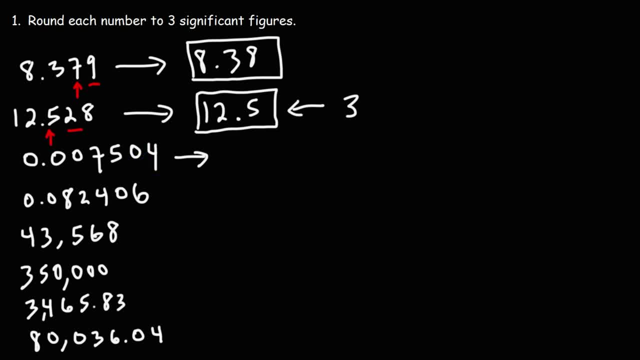 What would you say? Well, 4.. It's not 5 or more, so we're going to round this down Now. should we write the answer as .0075? Or should we write it as .00750?? What would you say? 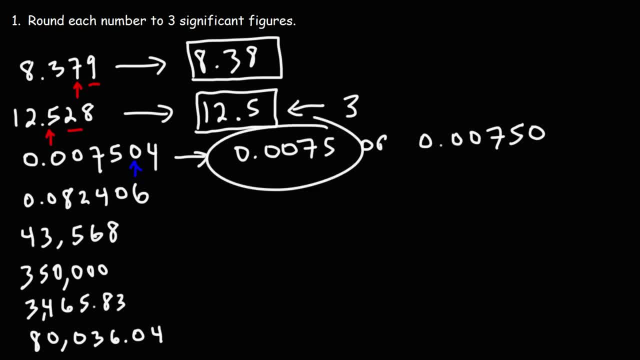 Looking at this number, that's two significant figures, So that wouldn't fit what we're trying to do here. This zero to the right Of a non-zero digit is significant if there's a decimal point. Again, if you want to learn these rules, check out that video. Significant Figures. a fast review. 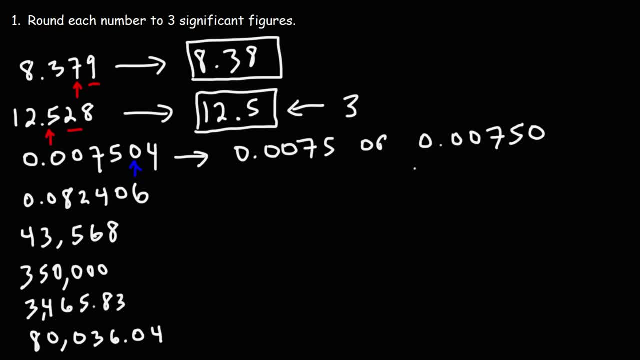 So, because this zero is significant, this is the answer. It has three significant figures. Now, moving on to the next example, we have .082406.. So the four is the third significant digit from the left. Looking at the next one, the zero that tells us we need to round down. 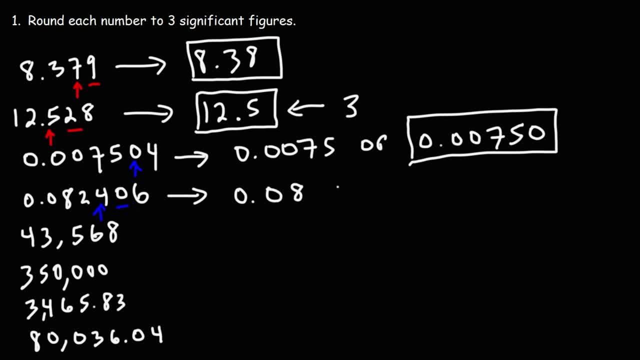 So we're just going to make this .0824.. Now, what about 43,568?? What should we do with such a large number? Well, we're going to follow the same process. We're going to look at the third significant. 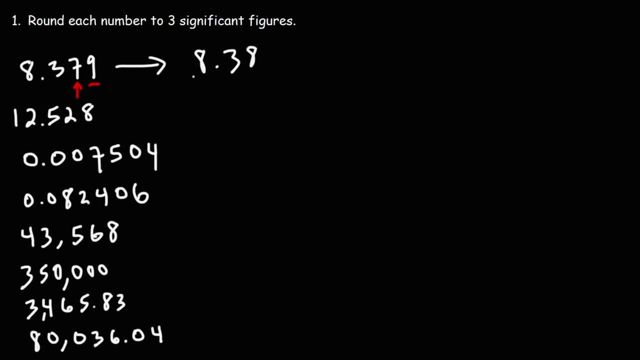 So this is going to be 8.38.. And this number has three sig figs, so we could stop here. Now, what about 12.528?? So we're going to focus on the third significant digit. Looking at the 2, that tells us that we need to round down. 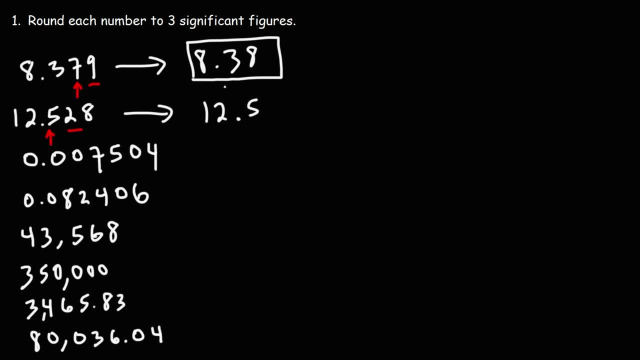 So we're going to round 12.528 to 12.5.. So this number has three sig figs. Now what about .007504?? Now you need to know that zeros to the left of the first significant digit, these zeros are not significant. 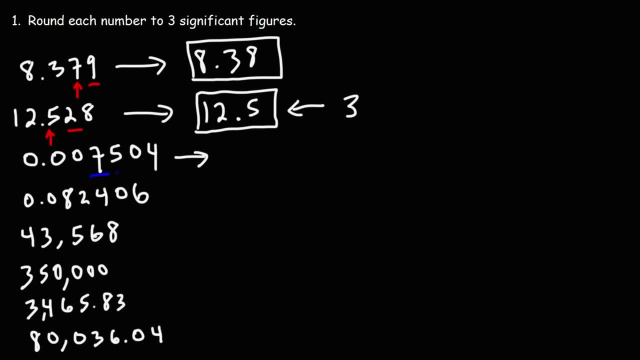 So this is the first significant digit. this is the second one. A zero between two non-zero numbers. that zero is significant, So this zero is the third significant digit counted from the left. So we need to focus on this one. Looking at the number 4, should we round this number down to zero or round it up to 1?? 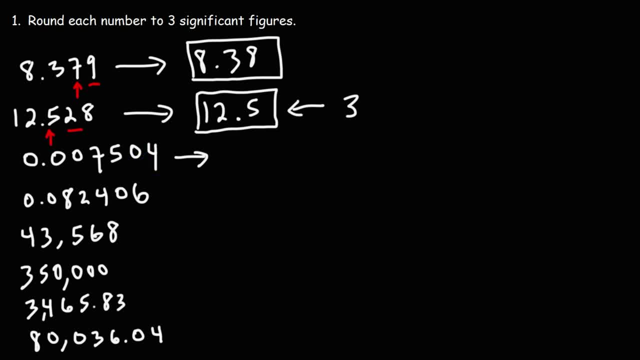 What would you say? Well, 4.. It's not 5 or more, so we're going to round this down Now. should we write the answer as .0075? Or should we write it as .00750?? What would you say? 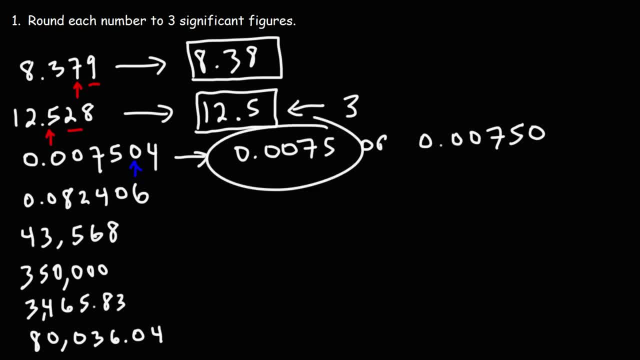 Looking at this number, that's two significant figures, So that wouldn't fit what we're trying to do here. This zero to the right Of a non-zero digit is significant if there's a decimal point. Again, if you want to learn these rules, check out that video. Significant Figures. a fast review. 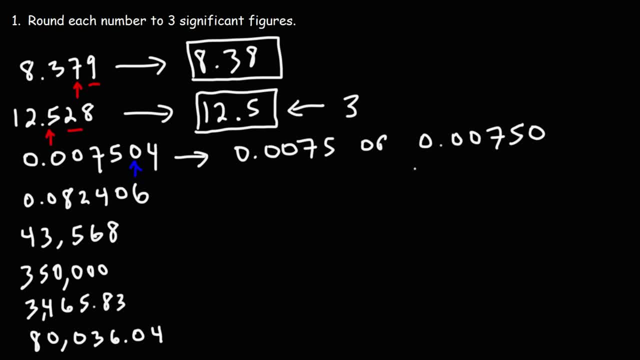 So, because this zero is significant, this is the answer. It has three significant figures. Now, moving on to the next example, we have .082406.. So the 4. Is the third significant digit from the left. Looking at the next one, the zero that tells us we need to round down. 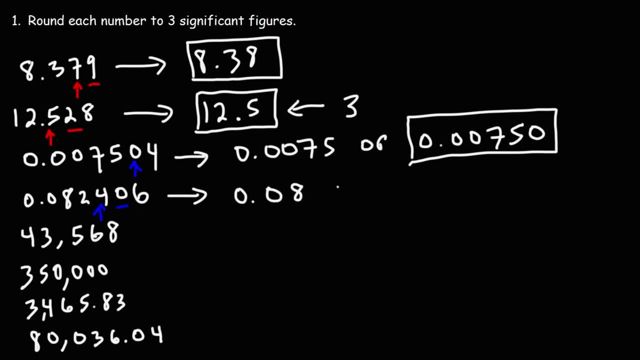 So we're just going to make this .0824.. Now, what about 43,568?? What should we do with such a large number? Well, we're going to follow the same process. We're going to look at the third significant digit. 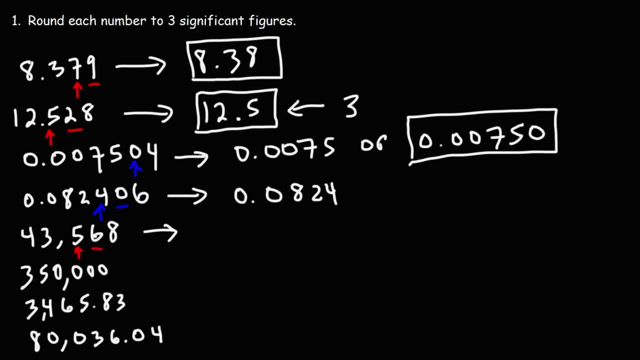 We're going to look at the fourth significant digit and we're going to focus on the number to the right. So, because we have a six which is five or more, we're going to round this number up. So here we have 568.. 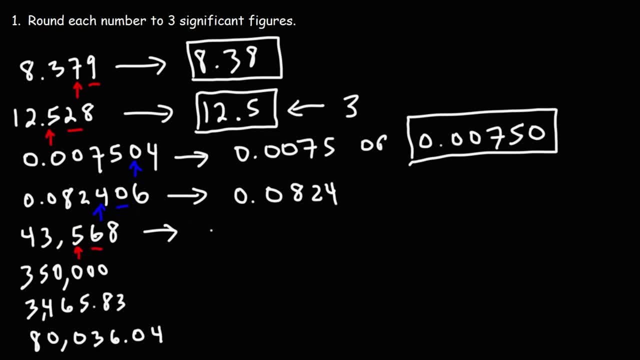 We're going to round that five to a six, But the question is, how should we write this After we write 43 and then six? what should we do after that? Because if we leave it as 436.. 436 has a, it's significantly different in value compared to 43,568.. 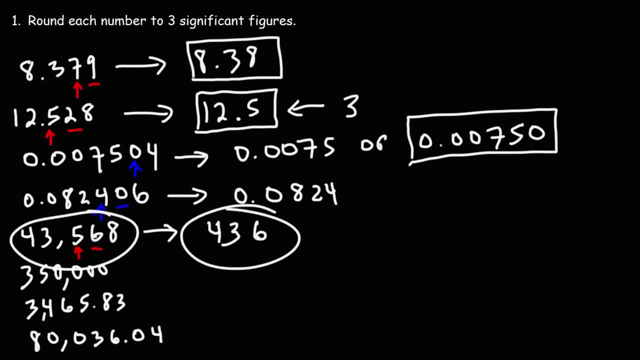 So we can't stop here, because these two numbers are nowhere close to each other. In a situation like this, you need to replace these numbers with a zero, So 568,. you want to round that up to 600.. So this becomes 43,600.. 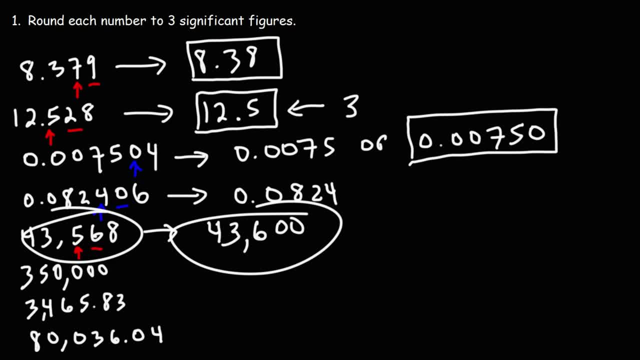 These two numbers are much closer to each other And we have three significant figures, The zeros to the right of six. they're not significant because we do not have a decimal point. So because we have three sig figs, we can leave the answer like this: 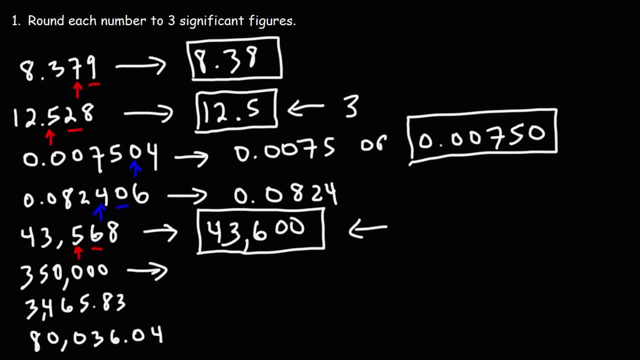 Now what about 350,000?? This one could be a little tricky. How would you round this to three sig figs? I want you to take a moment to Think about this one, to figure it out. So if we focus on the third significant figure, you may think it's a zero, but that zero is not significant. 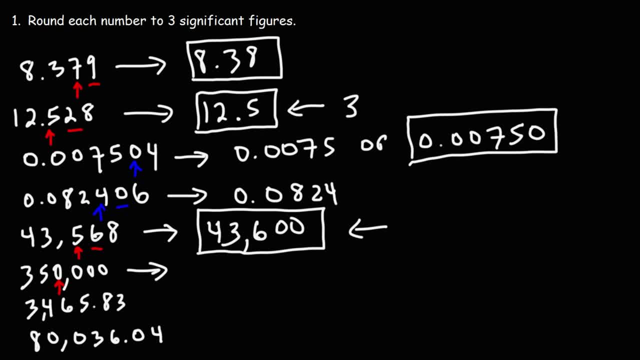 Because we don't have a decimal point and it's not between two non zero digits, the same way as this zero is not significant. So how can we round this to three sig figs? Would you focus on the five? If you focus on the five and look to the zero, you would have to round the five down or keep it at a five. 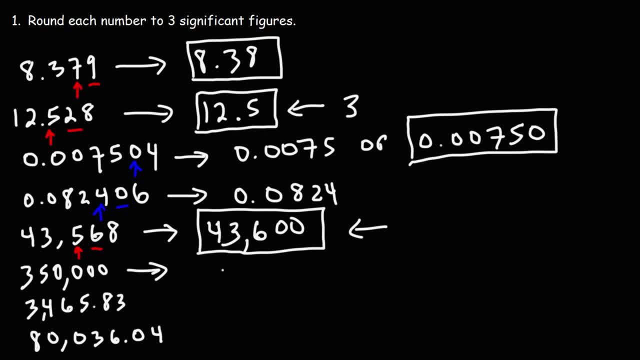 So what would you do here? In a situation like this, it's easier if you convert this to scientific notation. By the way, for those of you who haven't learned how to convert a number like this to scientific notation, I'm going to put some links in the description below. 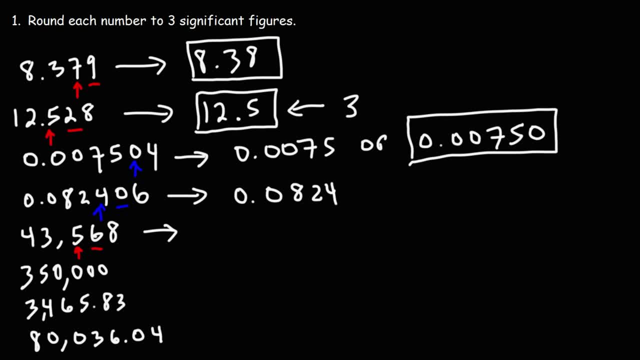 And we're going to focus on the number to the right. So, because we have a 6,, which is 5 or more, we're going to round this number up. So here we have 568.. We're going to round that 5 to a 6.. 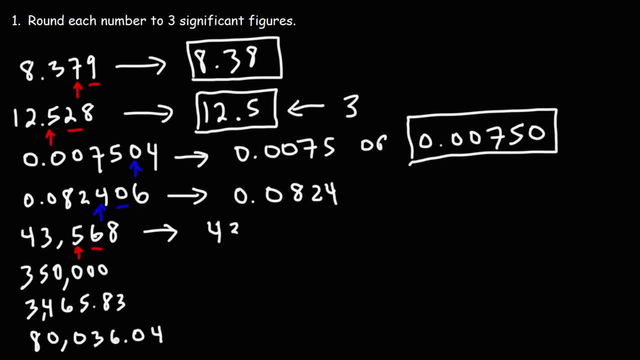 But the question is, how should we write this After we write 43 and then 6,? what should we do after that? Because if we leave it as 436, 436 has a. It's significantly different in value compared to 43,568.. 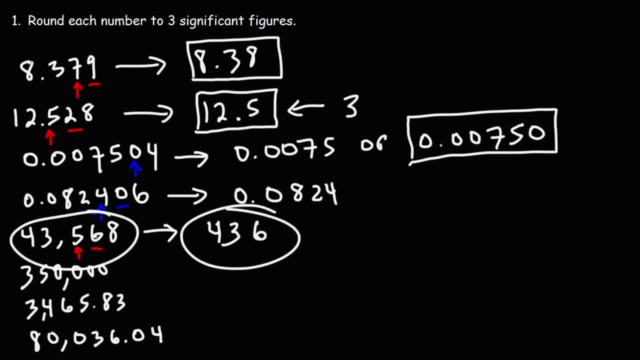 So we can't stop here, because these two numbers are nowhere close to each other. In a situation like this, you need to replace these numbers with a zero, So 568,. you want to round that up to 600.. So this becomes 43,600.. 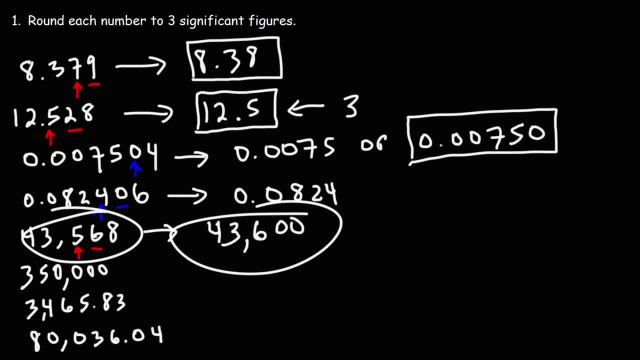 These two numbers are much closer to each other And we have Three significant figures, The zeros to the right of 6,. they're not significant because we do not have a decimal point. So because we have three sig figs, we can leave the answer like this: 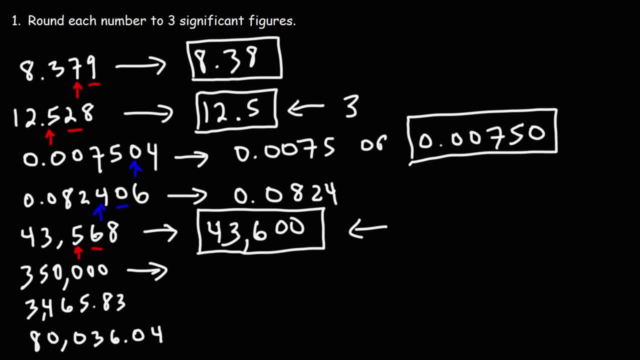 Now what about 350,000?? This one could be a little tricky. How would you round this to three sig figs? I want you to take a moment to think about this one, to figure it out. So if we focus on the third significant figure, you may think it's a zero, but that zero is not significant because we don't have a decimal point. 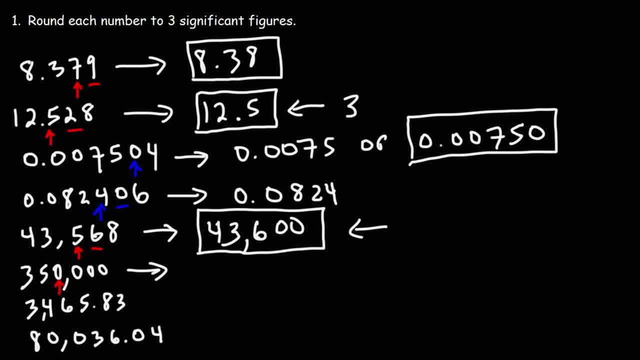 And it's not between two non-zero digits. The same way as this zero is not significant. So how can we round this to three significant figures? Would you focus on a five? If you focus on a five and look to the zero, you would have to round the five down or keep it at a five. 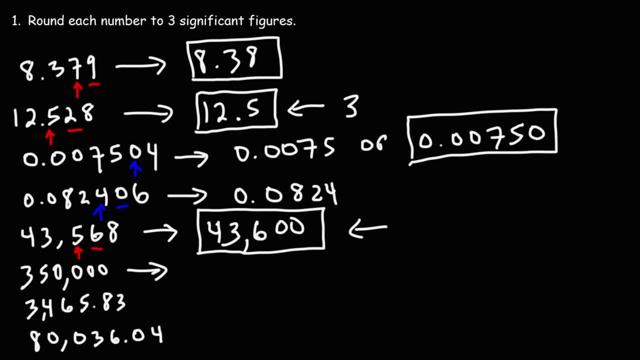 So what would you do here In a situation like this? it's easier if you convert this to scientific notation. By the way, for those of you who haven't learned how to convert a number like this to scientific notation, I'm going to put some links in the description section below. 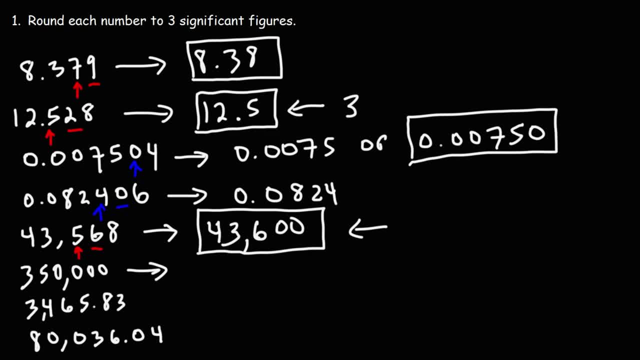 That will explain how to do that. But here's the quick shortcut method. If we were to add a decimal point here, to convert it to scientific notation we need to move the decimal point between the first two non zero digits- So one, two, three, four, five or correction- between the first two digits. 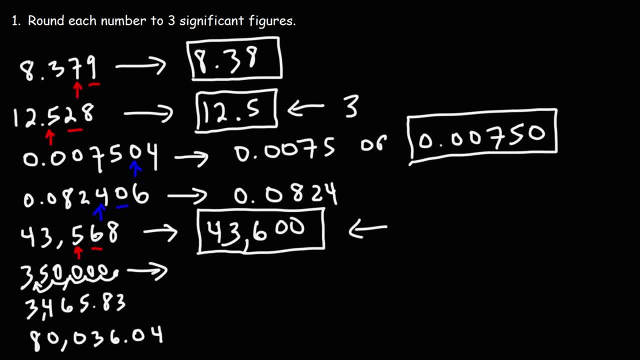 That's more accurate way of describing it. So basically we need to get the decimal point here. So we're going to go to the first two digits. That's more accurate way of describing it. That's my point here. Because we move it five spaces to the left, this is going to become 3.5.. 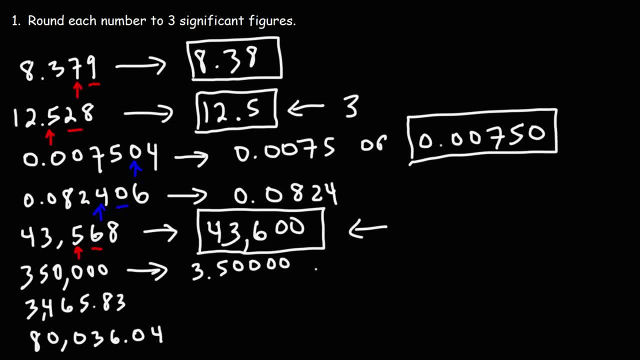 I'm going to keep all the zeros for now. We had four zeros and we moved five spaces to the left, So this is going to be 10 to the fifth power, 10 to the fifth power. If you multiply 10 five times, you're going to get 100,000. 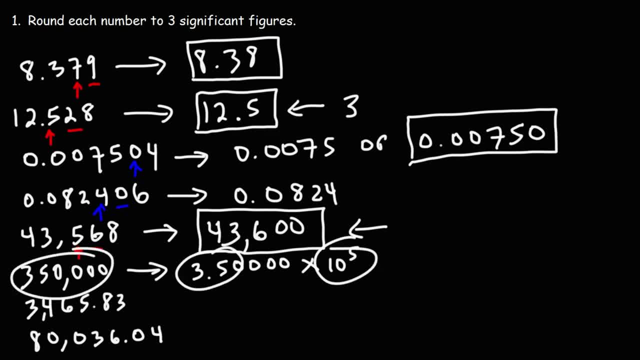 And 3.5 times 100,000 is 350,000.. So you could check your work by doing a quick mental calculation. But right now we have our number in scientific notation. But at this point all these zeros are considered significant because we have a decimal point. 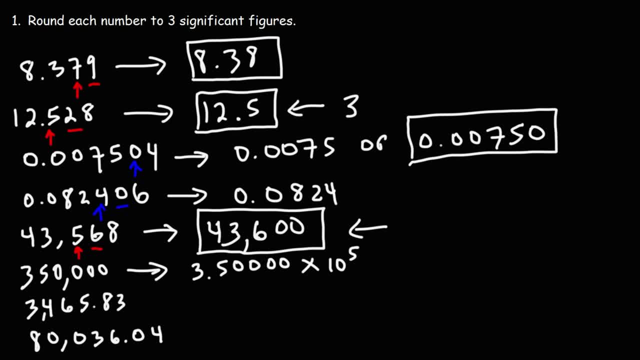 So, in order to run into three significant figures, we need to get rid of some zeros. All we got to do is just get rid of these three zeros and we're good. So the answer is going to be 3.50 times 10 to the five. 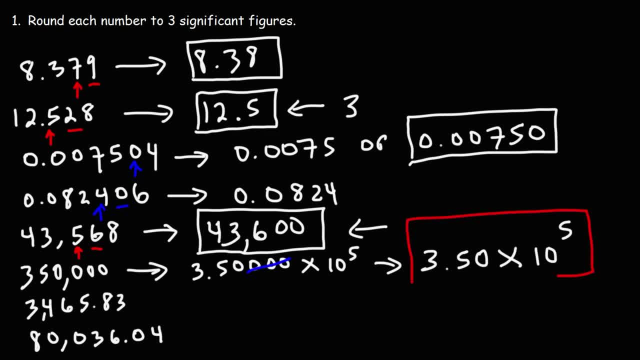 So now let's check our answer. This answer has three sig figs, three significant figures, three, five and zero, And at the same time it's exactly equal to the original number, which is great. So once those two criteria are met, where you have the appropriate significant figures and this number is either exactly equal or very close to in value, then you know you've done it correctly. 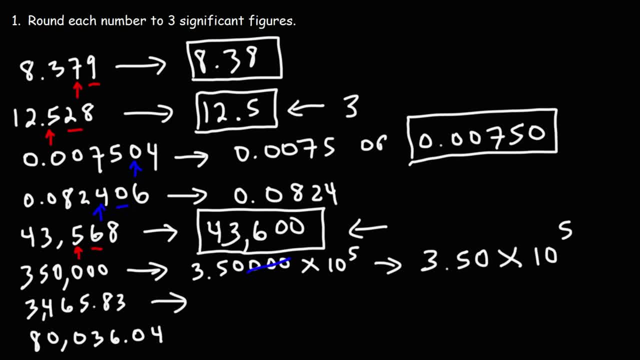 Now, moving on to the next example, we have 3,465.83.. Let's round that to three significant figures. So we're going to focus on the third significant digit, which is a six. Looking at the number to the right, that's a five. 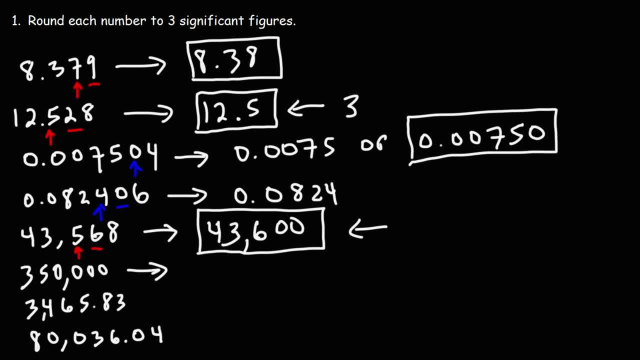 So if you're interested in learning how to convert a number like this to scientific notation, that'll explain how to do that. But here's the quick shortcut method. If we were to add a decimal point here to convert it to scientific notation, 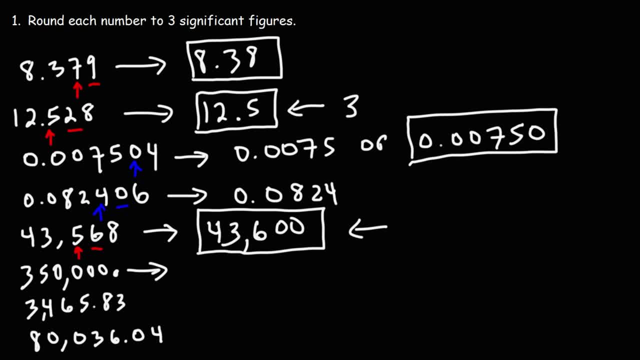 we need to move the decimal point between the first two non-zero digits, So one, two, three, four, five Or a correction, between the first two digits. That's a more accurate way of describing it. So basically, we need to get the decimal point here. 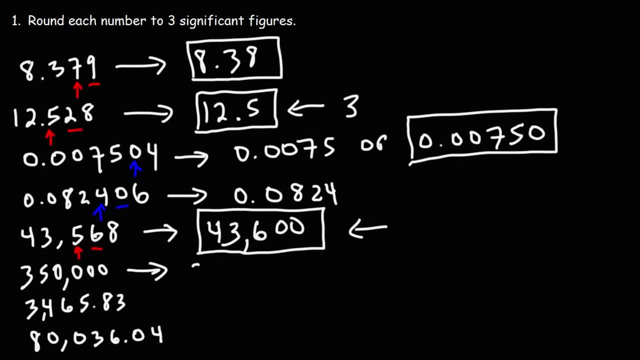 Because we move it five spaces to the left. this is going to become 3.5.. I'm going to keep all the zeros for now. We had four zeros And we moved five spaces to the left, so this is going to be 10 to the fifth power. 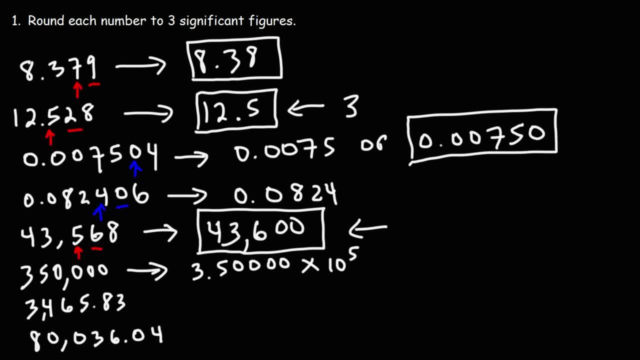 10 to the fifth power. if you multiply 10 five times, you're going to get 100,000.. And 3.5 times 100,000 is 350,000.. So you could check your work by doing a quick mental calculation. 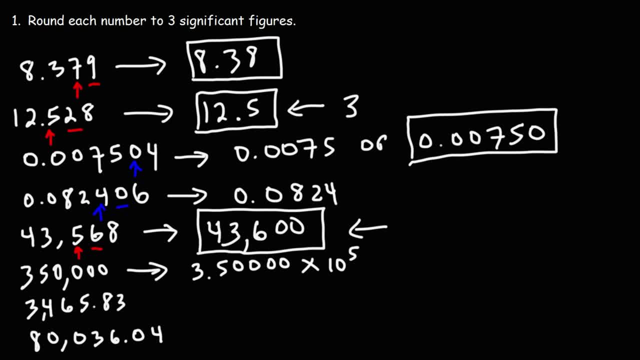 But right now we have our number in scientific notation, but at this point all these zeros are considered significant because we have a decimal point. So in order to round it to three significant figures, we need to get rid of some zeros. 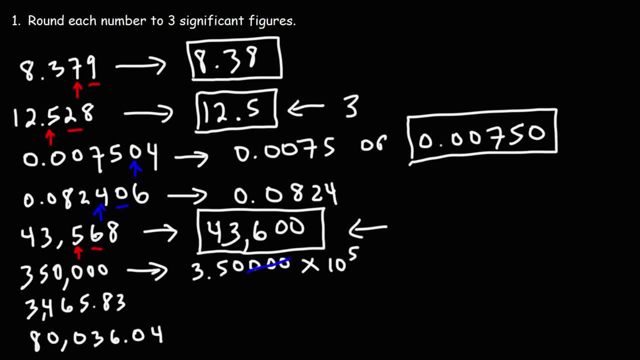 All we got to do is just get rid of these three zeros and we're good. So the answer is going to be 3.50 times 10 to the 5.. So now let's check our answer. This answer has three sig figs. 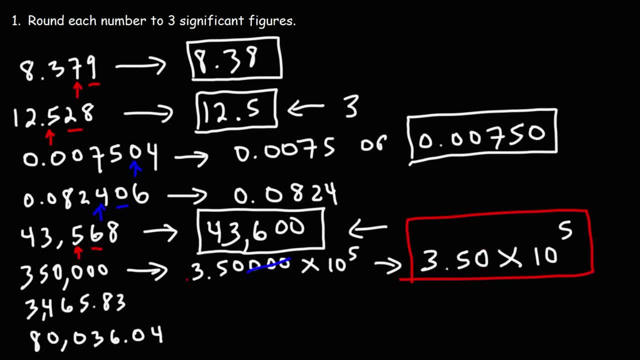 three significant figures- three, five and zero- And at the same time, it's exactly equal to the original number, which is great. So once those two criteria are met, where you have the appropriate significant figures and this number is either exactly equal or very close to in value, 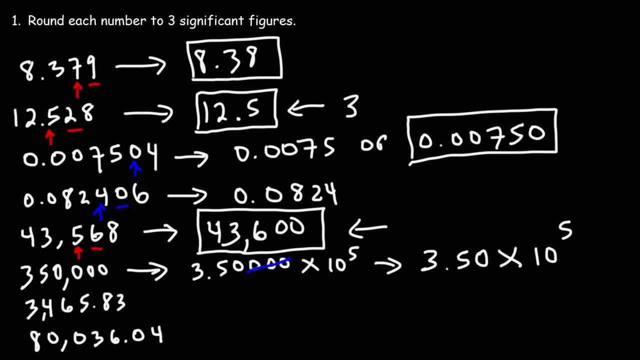 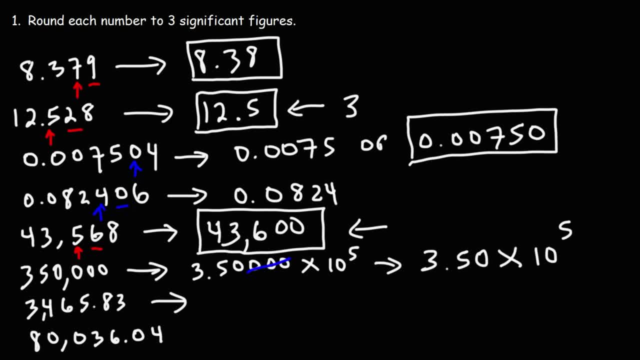 So we have 3,465.. Point 83.. Let's round that to three significant figures. So we're going to focus on the third significant digit, which is a six. looking at the number to the right, That's a five. 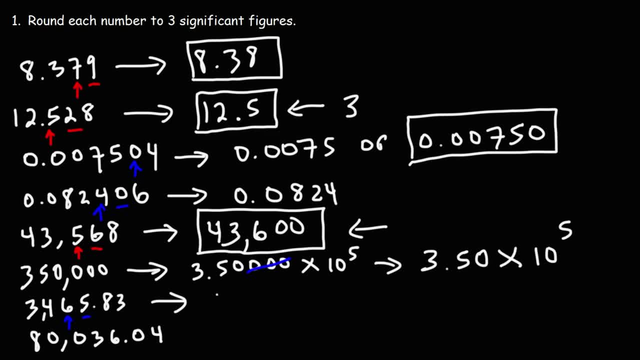 So we need to round the six up to a seven. So we're gonna have a three, a four and a seven. But what did we do here after that? Cuz 347 is nowhere close to three thousand 465.83.. 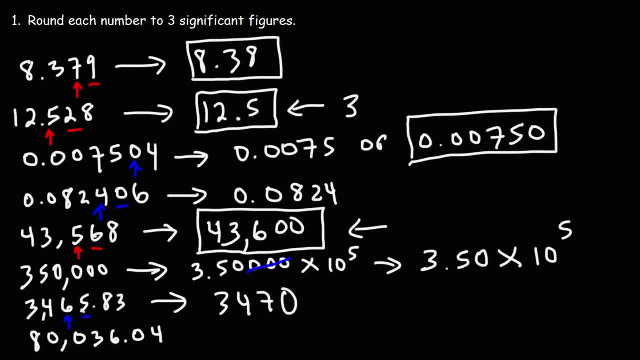 Now what we could do is add a zero. 3,465.83 is very close to 3,470.. And by adding a zero and not adding a decimal point, we already have three sig figs, So this answer is satisfactory. 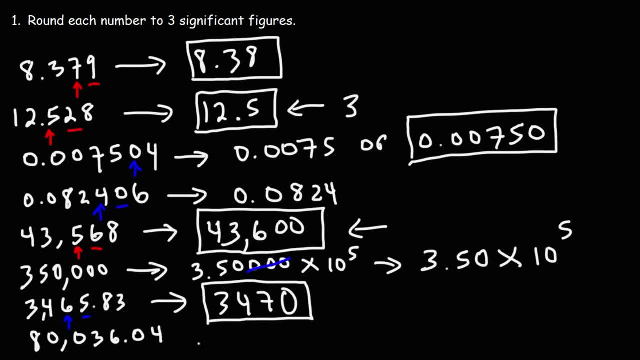 We can leave it like that. We don't have to convert to scientific notation, as in the case of the previous example. Now, moving on to the next one: 80,036.04.. What do we do here? So the zeros that are between non-zero digits, those are significant. 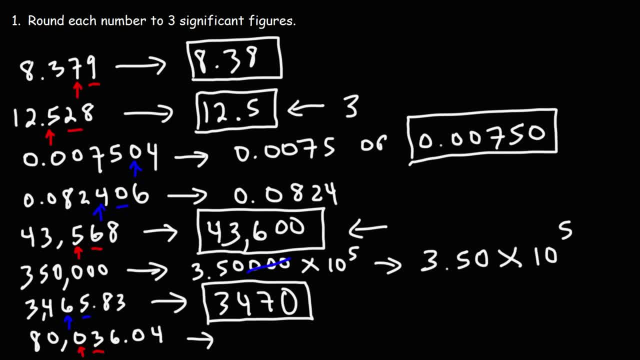 So this is the third significant figure And looking at the number to the right, that's a 3, so we're going to round down or we're going to keep it at a zero. So if we keep it zero or add a zero, we have 8,, 0, and a zero. 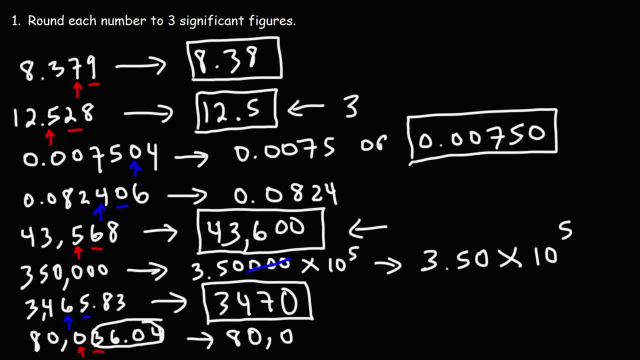 What do we do with these numbers here? Do we just change them all to zeros? If we did that, We could write it like this. or we could write it like this: If we were to write it as 80,000 without any decimal points, we would only have one significant figure. 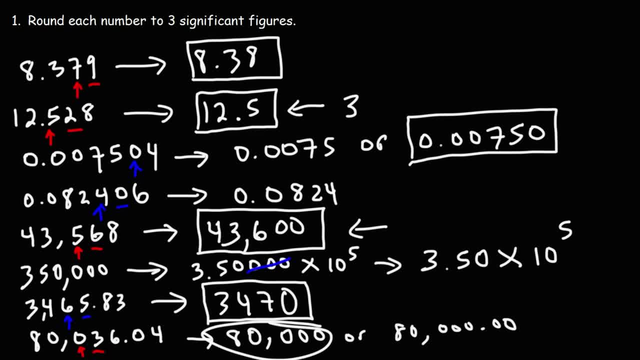 So we don't have three significant figures. therefore, this option is not going to work. Looking at this option, this will give us, Because of the decimal point, all the zeros are significant, So we would have 7. Significant figures. so that's not going to work. 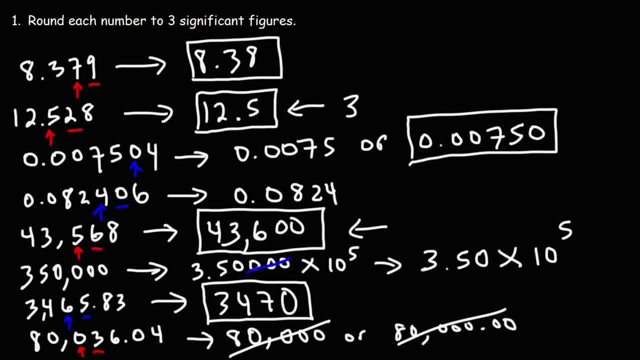 When you run into a wall like this, I recommend converting this into scientific notation. So let's move the decimal point between the first two numbers, So 1, 2, 3, 4.. As we move it four spaces to the left, we're going to get 10 to the 4.. 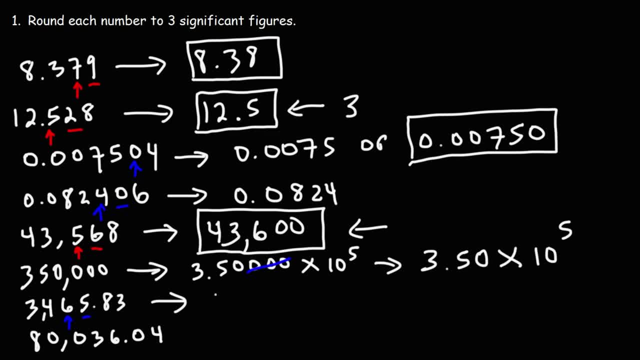 So we need to round the six up to a seven. So we're going to have a three, a four and a seven. But what do we do here after that? Because 347 is nowhere close to 3,465.. So we're going to have a three, a four and a seven. 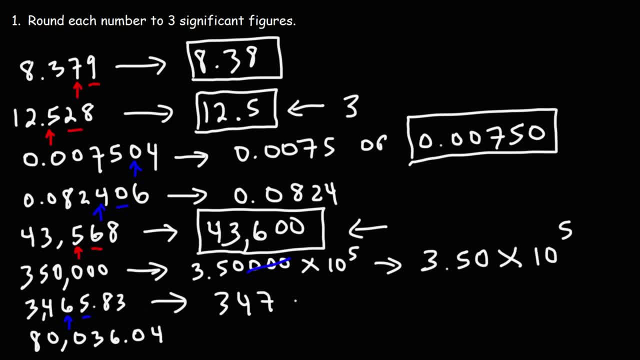 Now what we could do is add a zero. 3,465.83 is very close to 3,470.. And by adding a zero and not adding a decimal point, we already have three sig figs, So this answer is satisfactory. 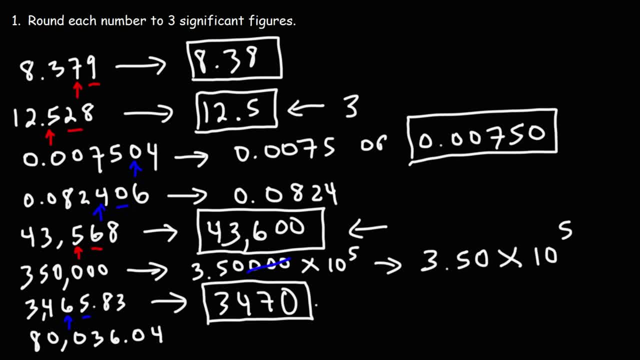 We can leave it like that. We don't have to convert to scientific notation, as in the case of the previous example. Now, moving on to the next one: 80,036.04.. What do we do here? So the zeros that are between non-zero digits, those are significant. 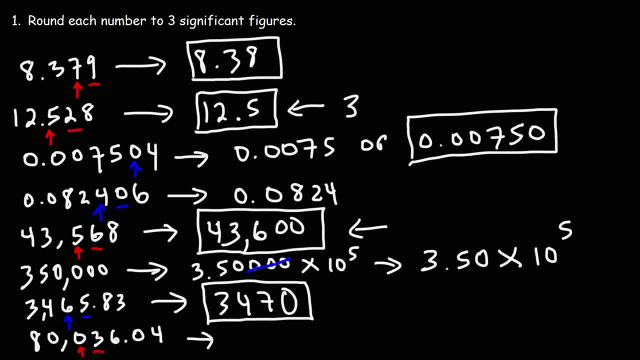 So this is the third significant figure And looking at the number to the right, that's a three. So we're going to round down or we're going to keep it at a zero. So if we keep it zero or add a zero, we have eight zero and a zero. 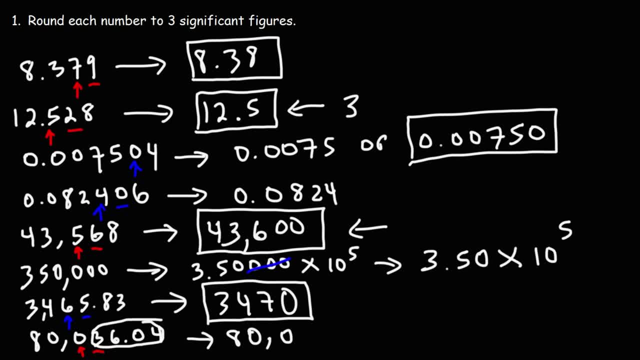 What do we do with these numbers here? Do we just change them all to zeros? If we did that, we could write it like this. or we could write it like this: If we were to write it as 80,000 without any decimal points, we would only have one significant figure. 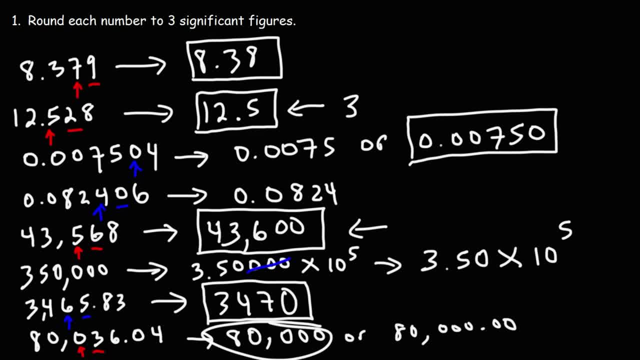 So we don't have three significant figures. Therefore, this option is not going to work. Looking at this option, This will give us, because of the decimal point, all the zeros are significant, So we would have seven significant figures. So that's not going to work. 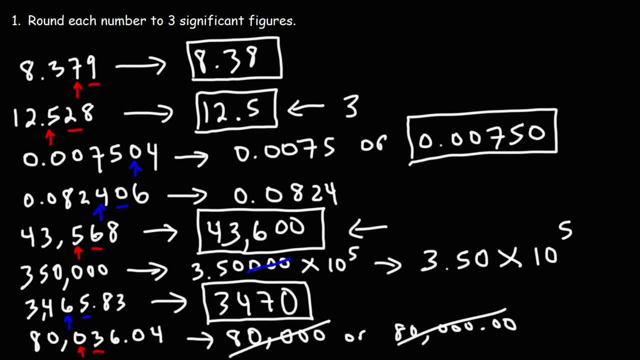 When you run into a wall like this, I recommend converting this into scientific notation. So let's move the decimal point between the first two numbers, So one, two, three, four. As we move it four spaces to the left, we're going to get ten to the fourth. 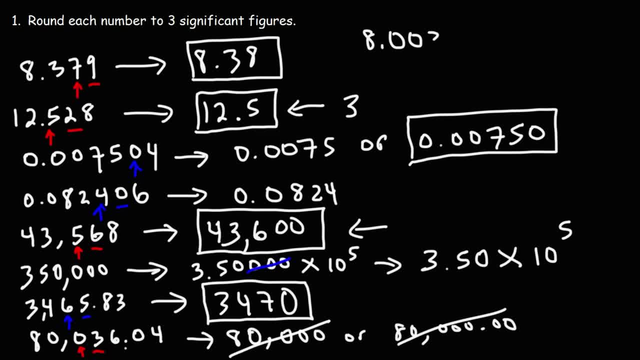 So this is eight Point zero, zero, three, six, zero, four times ten to the fourth. But right now we still have seven significant figures And we only want three. So we're going to keep this at a zero because of the next number, three. 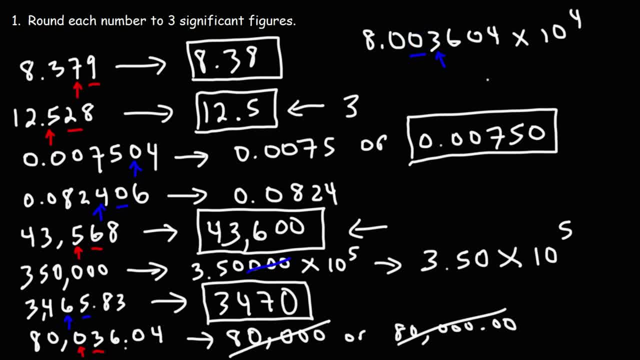 We need to round it down. So what we're going to do is we're going to convert this to eight, point zero, zero times ten to the fourth. Ten to the fourth is eight, So that's ten thousand. If you multiply ten four times times eight, that's approximately eighty thousand. 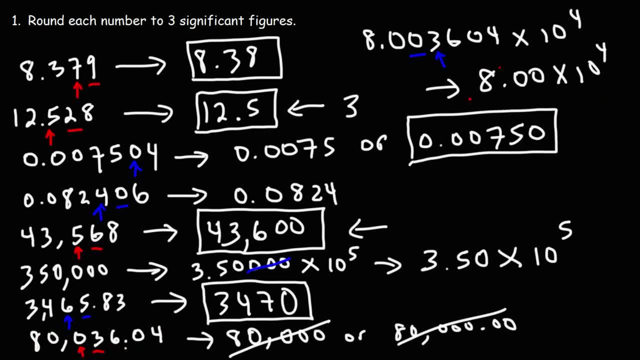 So these two are very close in value to each other, which is good, And we have three sig figs, which is also good. So this is going to be the best answer that we can come up with for this particular number. Now let's work on some more example problems. 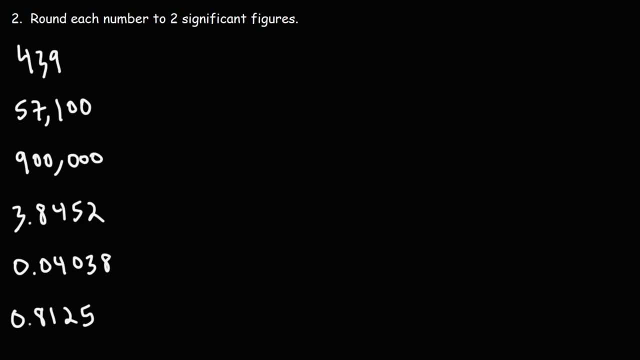 Round each number to two significant figures. So let's begin with four hundred thirty nine. Looking at the second significant digit, it's a three And the one to the right of that that's a nine. So we're going to round the three up. 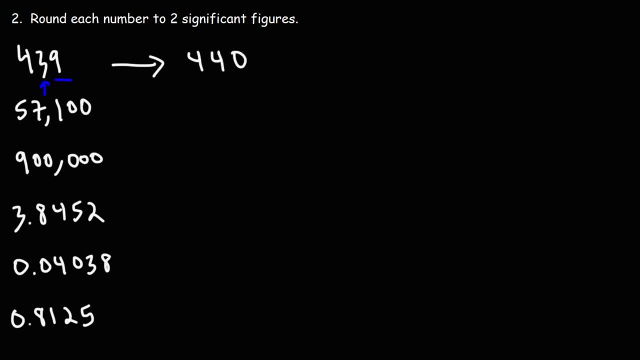 So from four hundred thirty nine we're going to round it to four forty. Now, if we were to put a decimal point, that would be three sig figs. So we're not going to do that. If we leave it like this, this zero is no longer significant. 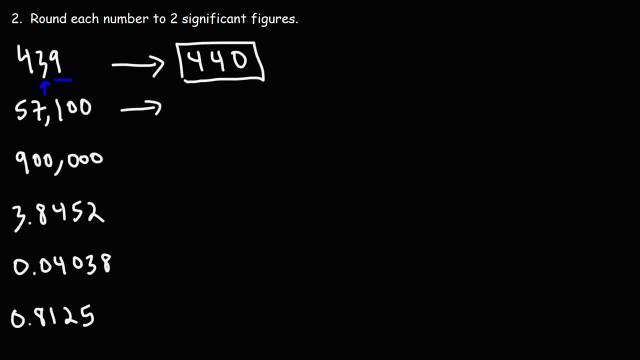 So we have two sig figs. So that's going to be the answer Now for the next one: fifty seven thousand one hundred. So looking at the second significant digit, it's a seven. To the right we have a one. 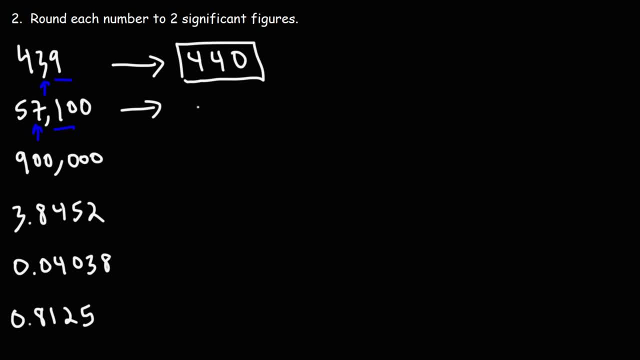 So we're going to round down So fifty seven thousand one hundred. we're just going to round that to fifty seven thousand Because, writing it this way, we have two significant figures And these two numbers are very close in value to each other. 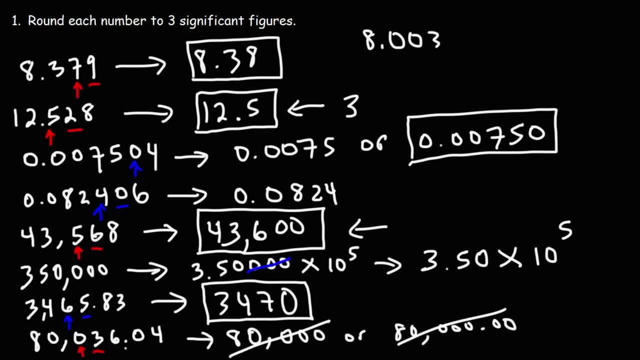 So this is 8.003604 times 10 to the 4.. Now we still have seven significant figures and we only want three. So we're going to keep this at a zero because, Because of the next number- 3, we need to round it down. 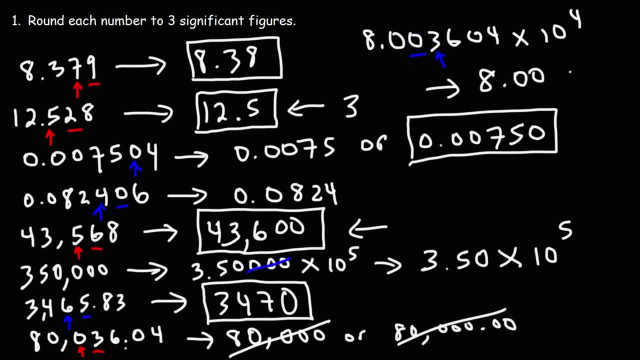 So what we're going to do is we're going to convert this to 8.00 times 10 to the 4.. 10 to the 4 is 10,000.. If you multiply 10 four times times 8, that's approximately 80,000.. 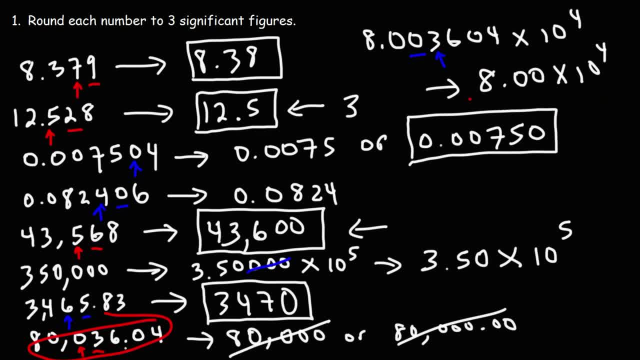 So these two are very close in value. They're very close in value to each other, which is good, And we have three sig figs, which is also good. So this is going to be the best answer that we can come up with for this particular number. 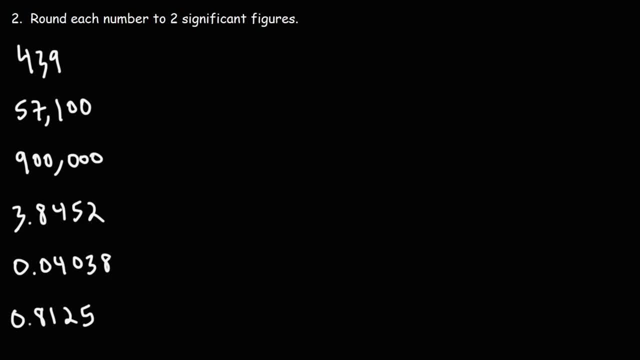 Now let's work on some more example. problems Round each number to two significant figures, So let's begin with 439.. Looking at the second significant digit, It's a three And the one to the right of that that's a nine. 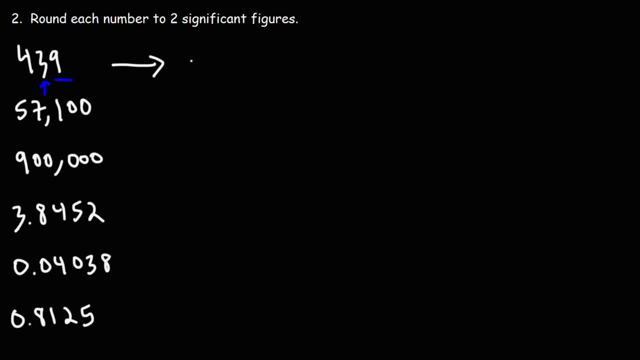 So we're going to round the three up. So from 439, we're going to round it to 440.. Now, if we were to put a decimal point, that would be three sig figs. So we're not going to do that. 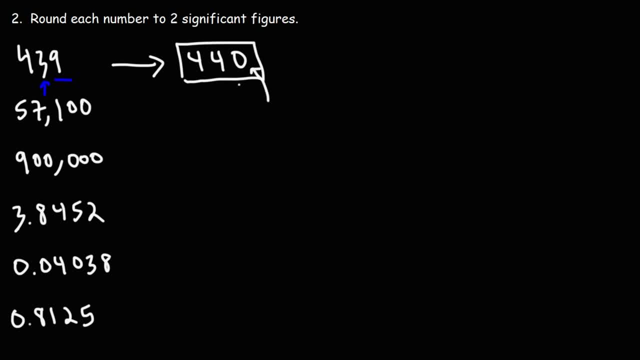 If we leave it like this, this zero is no longer significant. So we have two sig figs. So that's going to be the answer Now for the next one: 57,100.. So looking at the second significant digit, 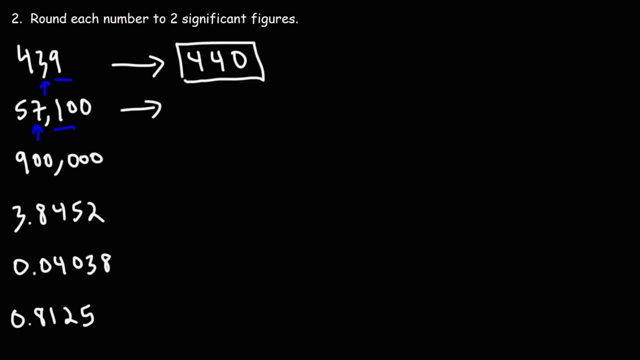 It's a seven to the right, We have a one, So we're going to round down So 57,100,. we're just going to round that to 57,000 because, writing it this way, we have two significant figures. 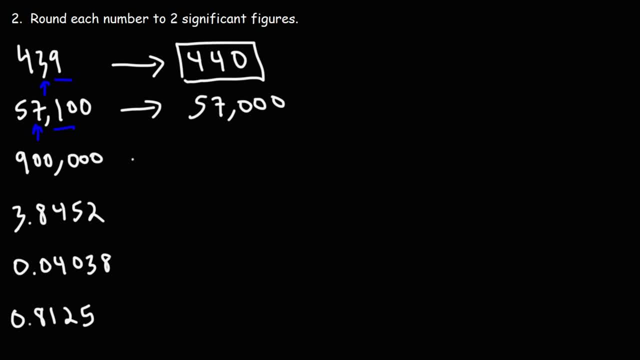 And these two numbers are very close in value to each other. Now what about the next one, 900,000.. How can we round that to two significant figures? What would you do here? In this case, it's good if we convert it into scientific notation. 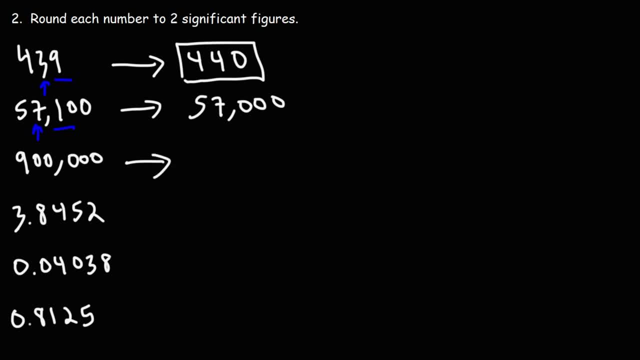 Now what about the next one? Nine hundred thousand. How can we round that to two significant figures? What would you do here? In this case, it's good if we convert it into scientific notation. So this will be nine point zero, zero, zero, zero, zero times ten to the five. 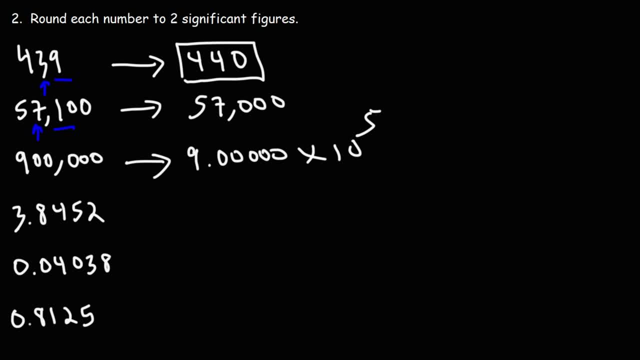 Ten to the five is a hundred thousand times nine. That gives us nine hundred thousand. But now we only want two significant figures, So we're going to get rid of the four zeros here. Therefore, we're going to leave our answer as nine point zero times ten to the five. 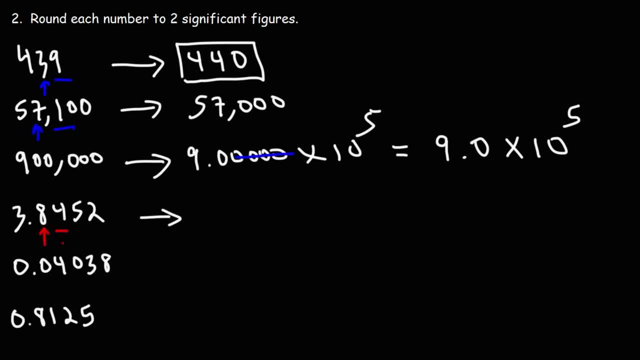 For the next one. looking at the four, that tells us we need to round down instead of up. So three point eight. four five, two becomes three point eight. Point zero, four, zero, three, eight. The second significant digit is a zero. To the right of that we have a three. so we're going to round down. 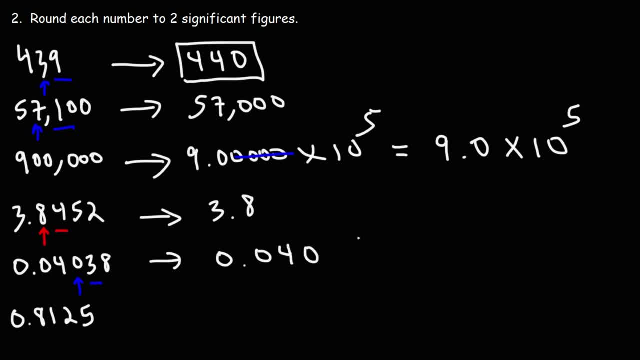 So we're going to round this to point zero, four zero. This zero is not significant, but this one is significant because of the decimal point. So what we have here is two significant figures. Now for point eight: one, two, five. this is the second significant digit. 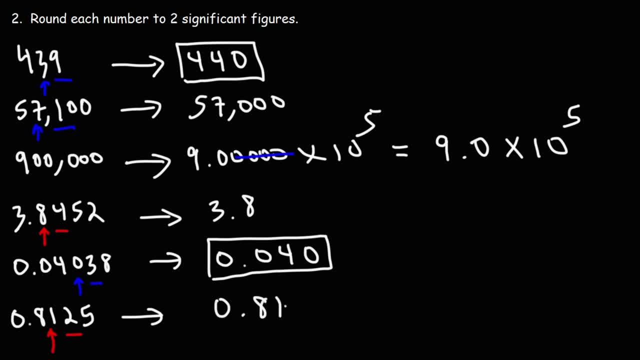 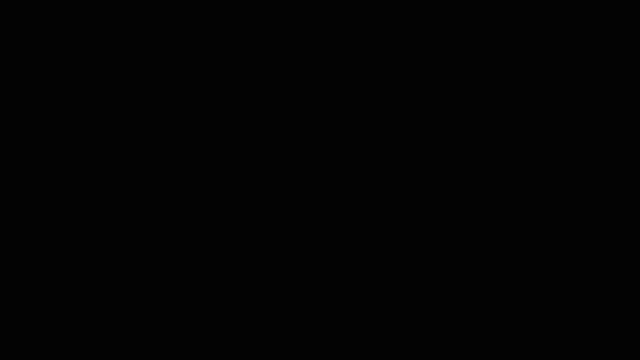 Looking at the two we need to round down, so we could just leave this as point eighty one. So that's it for this problem. Now for the next one. go ahead and round these numbers to one significant figure. So feel free to work on this as I write down these numbers. 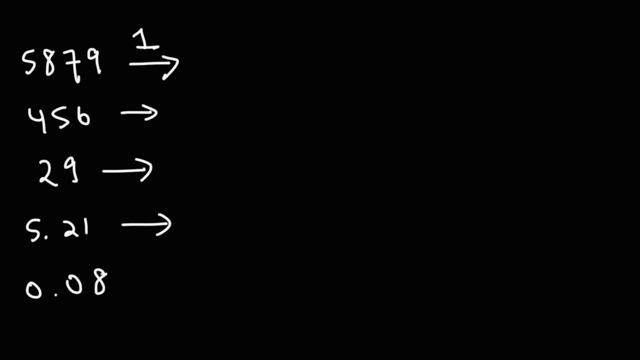 So fifty eight thousand, I mean five thousand, eight hundred seventy nine. If we want to round that number to one significant figure, we could just round it up to six thousand. Looking at the five, we see we have an eight which is five or more. 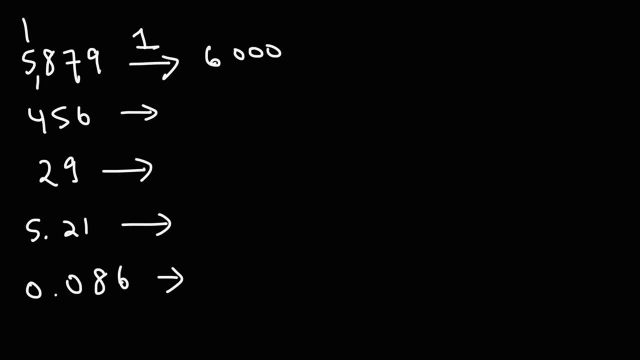 So we round the five up to a six. Six thousand is very close to five thousand eight hundred seventy nine. Now what about four? fifty six? How can we round that to one significant digit? So, focusing on the four, looking at the number to the right, we have a five. 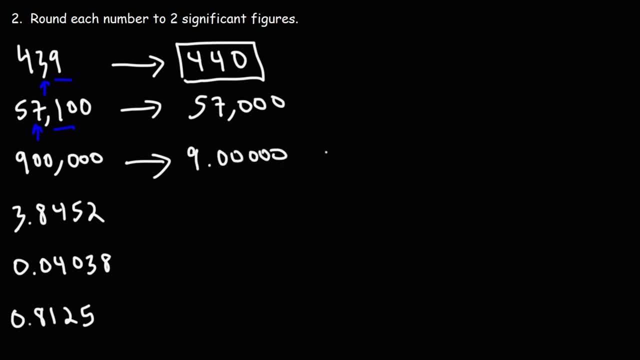 So this will be 9.000000 times 10 to the 5.. 10 to the 5 is 100,000 times 9.. That gives us 900,000.. But now we only want two significant figures, So we're going to get rid of the four zeros here. 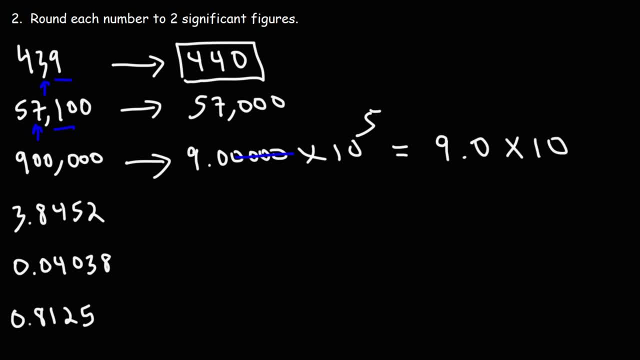 Therefore, we're going to leave our answer as 9.000.. 9.000 times 10 to the 5.. For the next one, looking at the four, that tells us we need to round down instead of up. So 3.8452 becomes 3.8.. 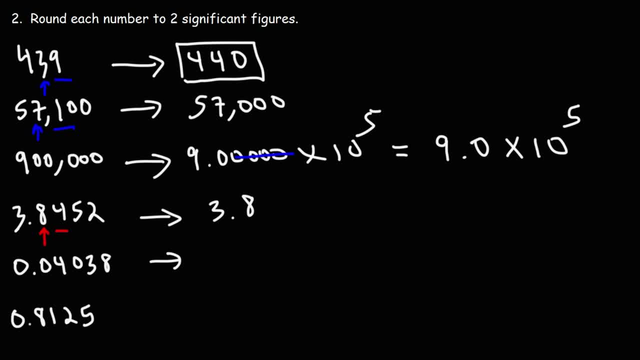 For 0.04038,. the second significant digit is a zero. To the right of that we have a three. So we're going to round down, So we're going to round this to 0.040.. This zero is not significant. 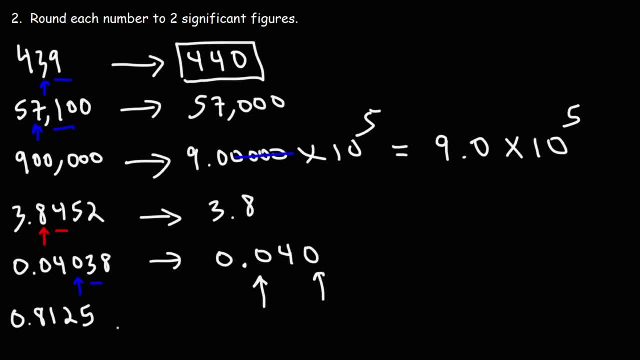 But this one is significant because of the decimal point. So what we have here is two significant figures. Now for 0.8125, this is the second significant digit, Looking at the two we need to round down, So we could just leave this as 0.81.. 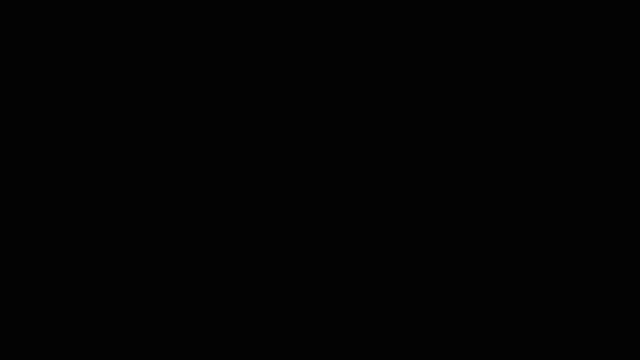 So that's it for this problem. Now for the next one. go ahead and round these numbers to 1.. One significant figure, So feel free to work on this as I write down these numbers. So 58,000, I mean 5,879.. 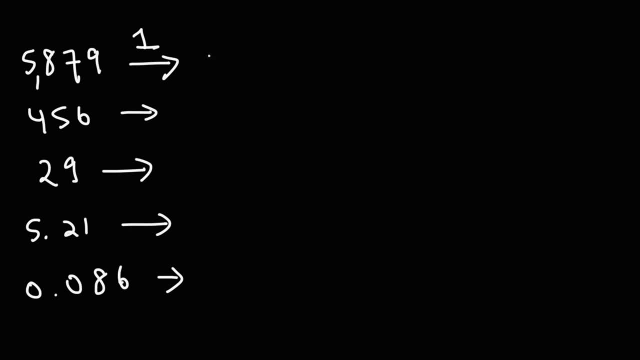 If we want to round that number to one significant figure, we could just round it up to 6,000.. Looking at the five, we see we have an eight which is five or more. So we round the five up to a six. 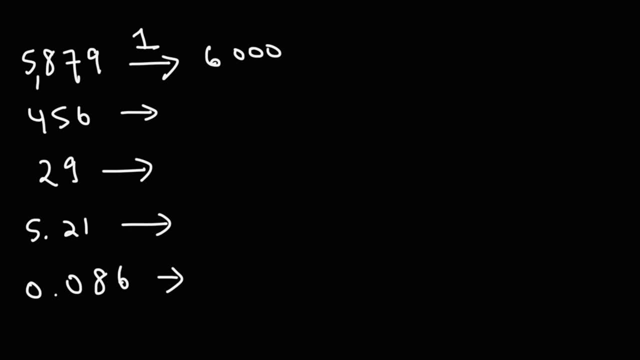 6,000 is very close to 5,879.. Now what about 456?? How can we round that to one significant digit? So, focusing on a four, looking at the number to the right, we have a five. We need to round the four up to a five. 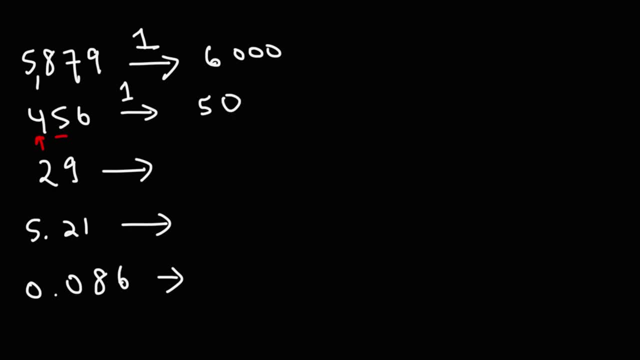 And then the other numbers, the five and six. we could just replace them with zeros, So 456.. we can round that up to 500.. Focus on the 2,. we have a 9 to the right, so we're going to round.